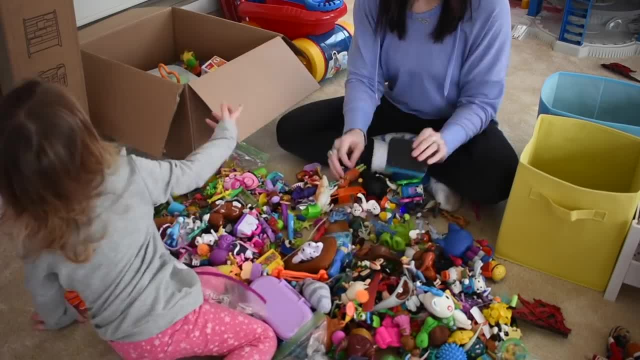 leave a comment below. I'll see you in the next video. Bye. Leave me a comment in the description box below If your kids have a lot of toys. if you're a minimalist- we are definitely obviously not minimalist, but I think it's. 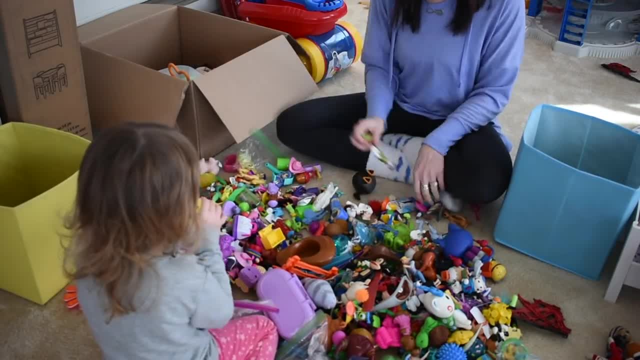 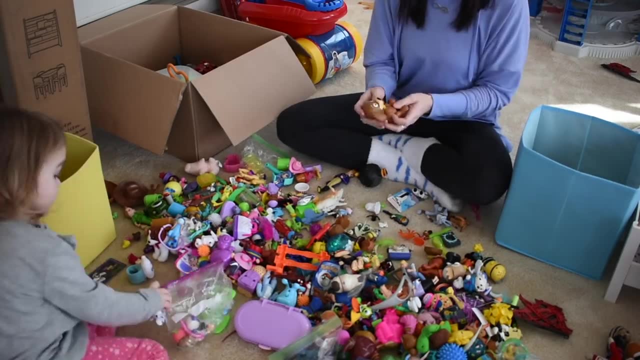 really fun that our kids have lots of options of toys in their toy room, So I really don't mind having this much. Sometimes it definitely becomes stressful but, like I said, it's not mine to get rid of And obviously we didn't buy everything for our children, so it's hard getting rid of. 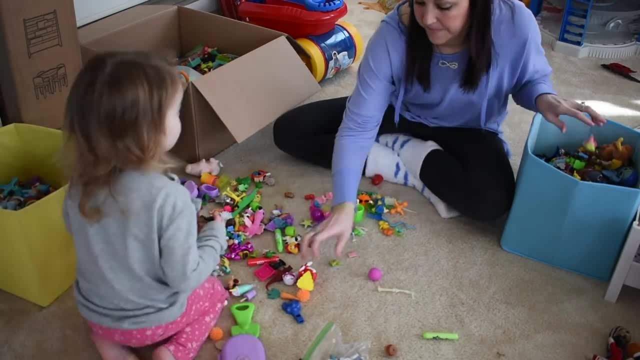 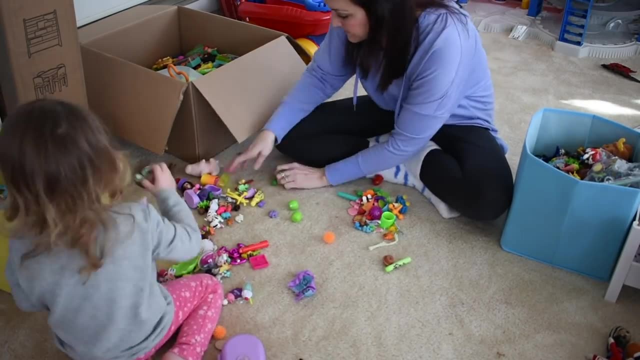 something that maybe their grandparents bought them. So if you guys do declutter your toy room with your children, I would love to hear from you in the comments below. So if you guys have, make sure you're very compassionate about it, because my kids' feelings get hurt so bad Maybe. 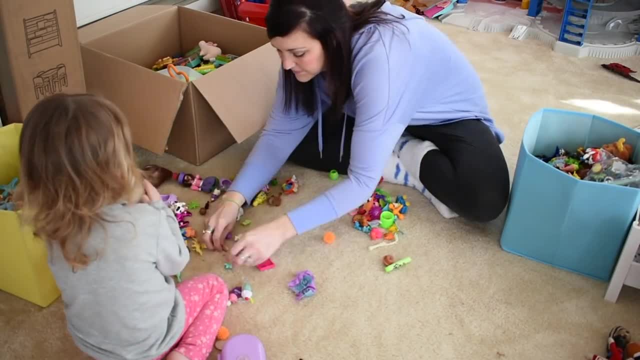 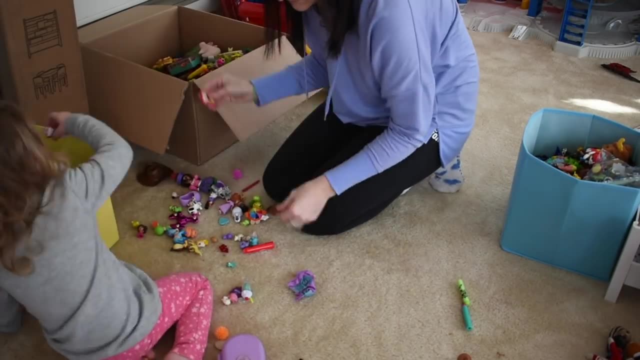 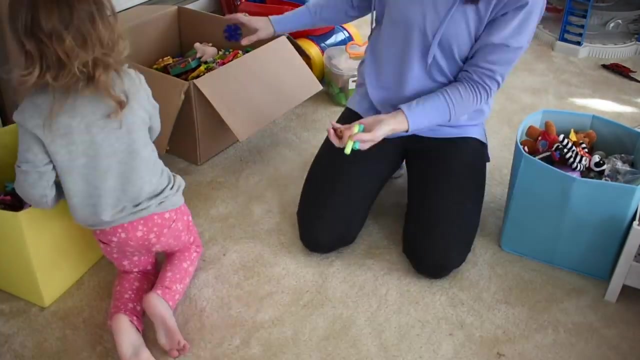 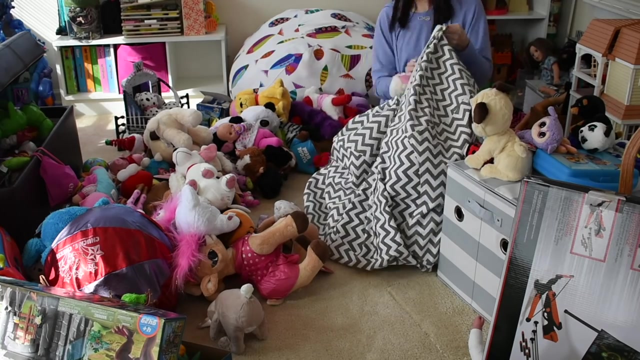 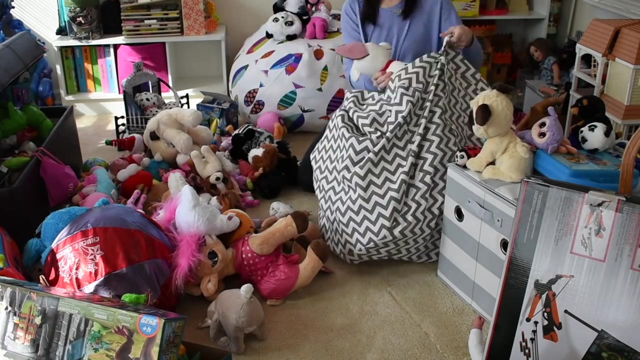 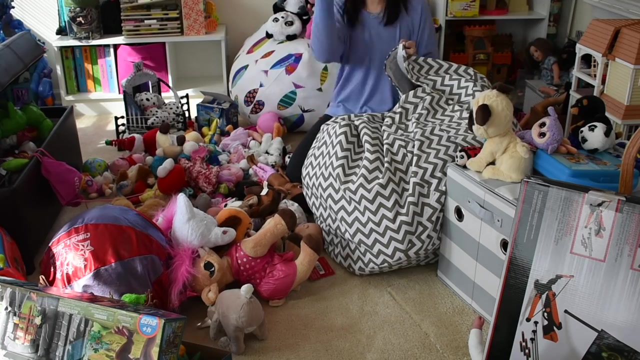 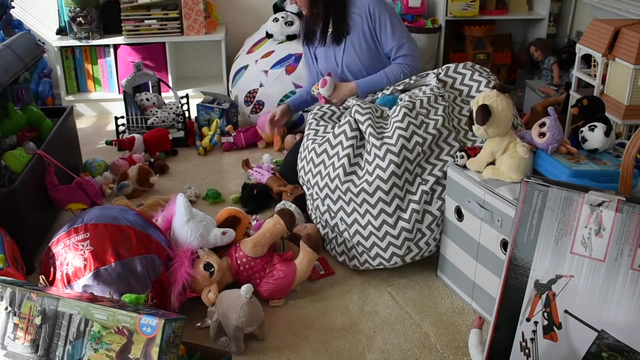 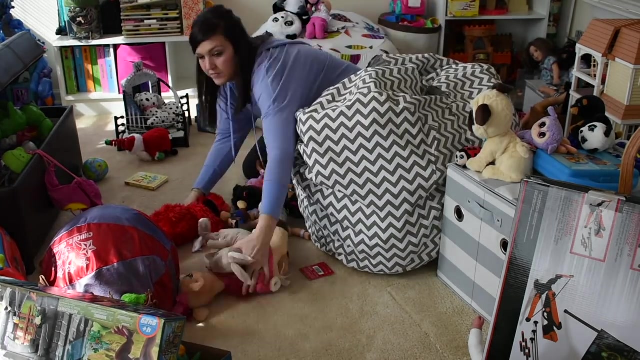 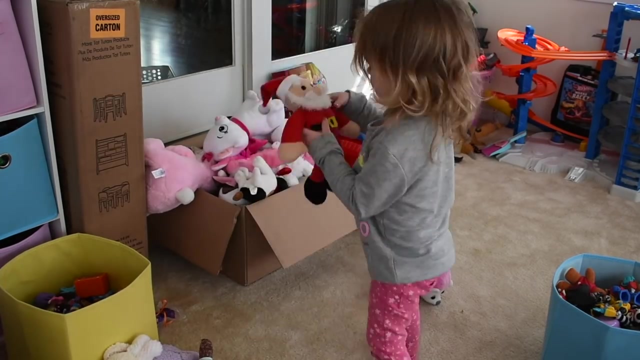 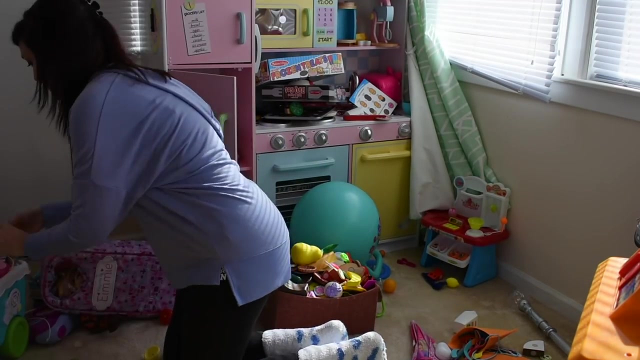 not yours, but mine do, And I really do care about their feelings and how they react to getting rid of things. But okay, done talking, Let's go. It's not about our love. It's not about I think I'm arsenic. 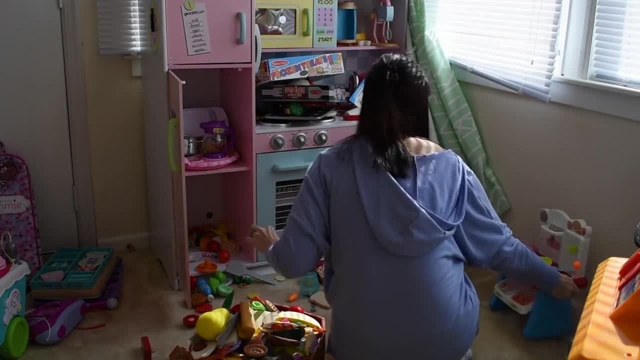 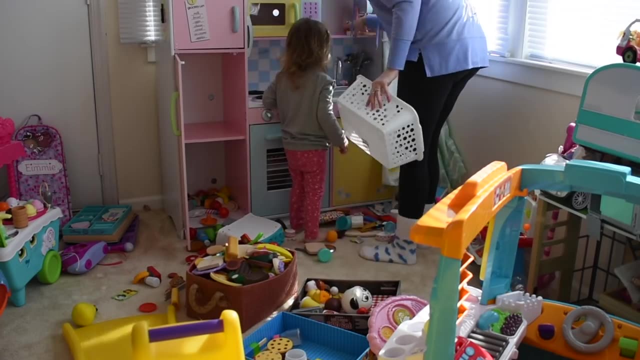 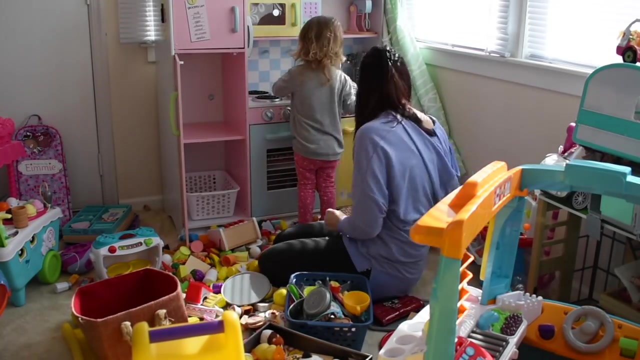 But you don't mind that I'm toxic. Somehow you're fine with it, Even when I'm chaotic. You see the shade in the cold. It's just my bad temper. What am I supposed to do When the flame's going high With my, my bad patience? 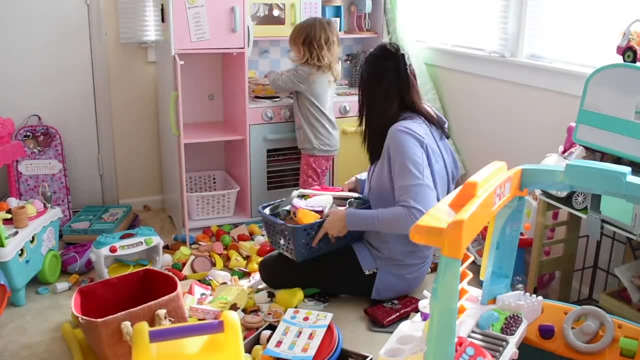 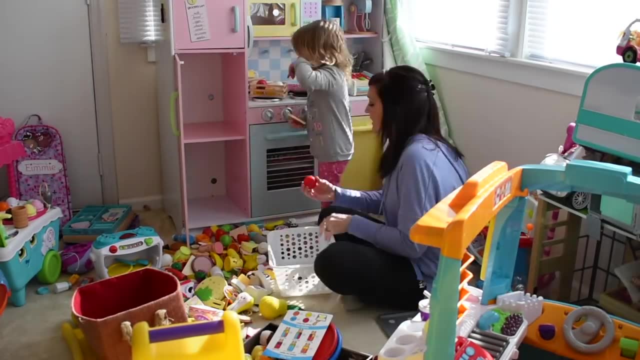 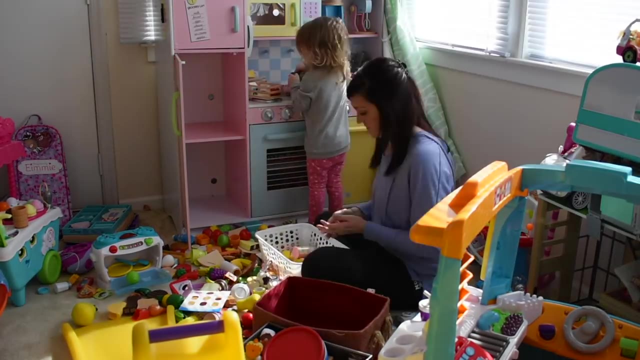 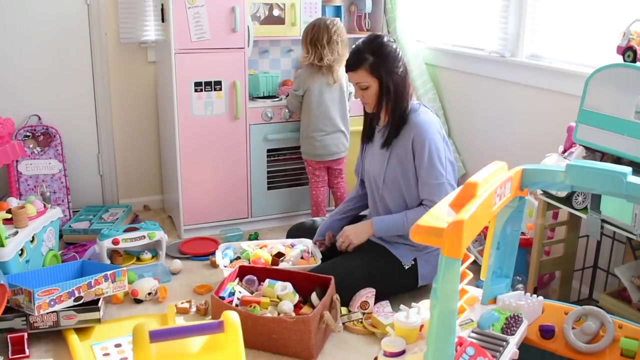 I hate it always falls on you, But you know it's not about our love fading. You know it's not about- Yeah, you know it's not about our love ending. You know it's not about. It's not about us. You know it's not about us. 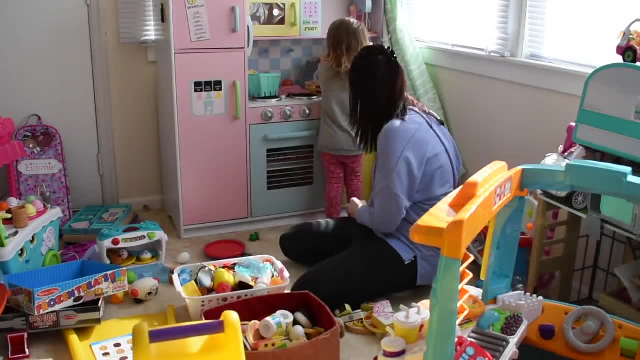 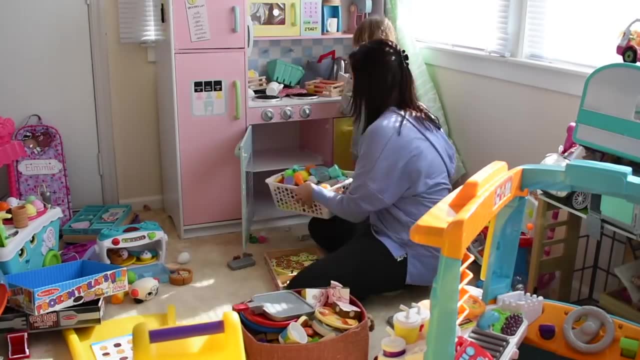 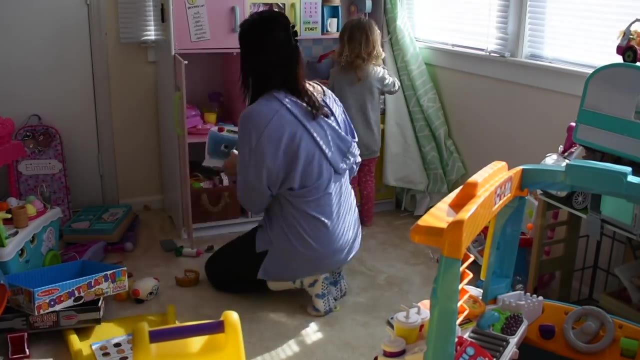 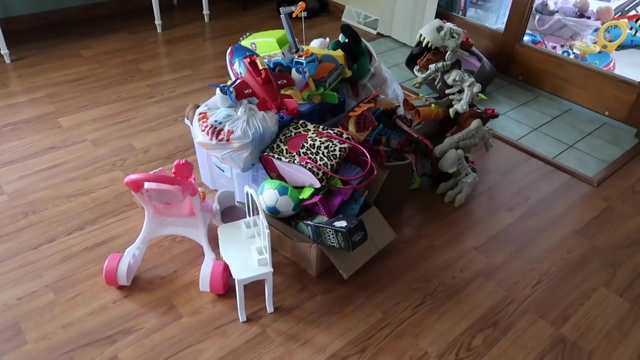 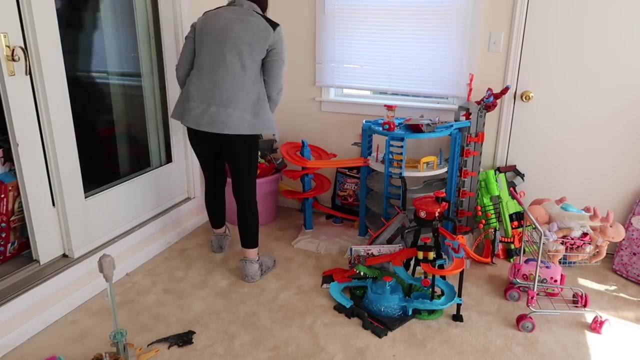 You know it's not about us. You know it's not about us. You see the shade in the cold. It's just my bad temper. What am I supposed to do When the flame's going high With my, my bad patience? I hate it always falls on you. 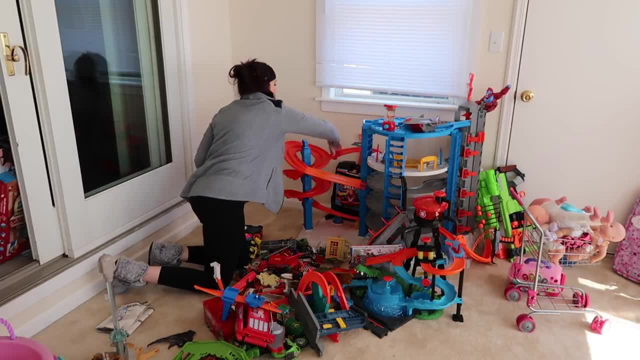 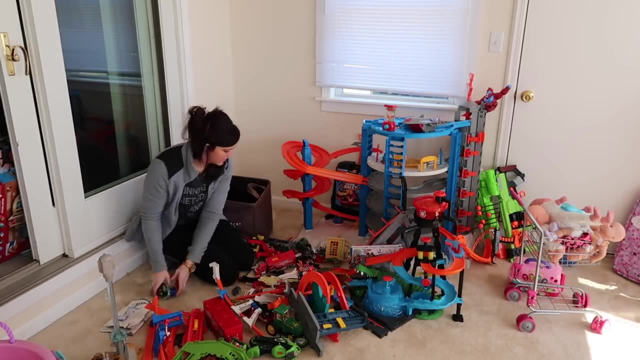 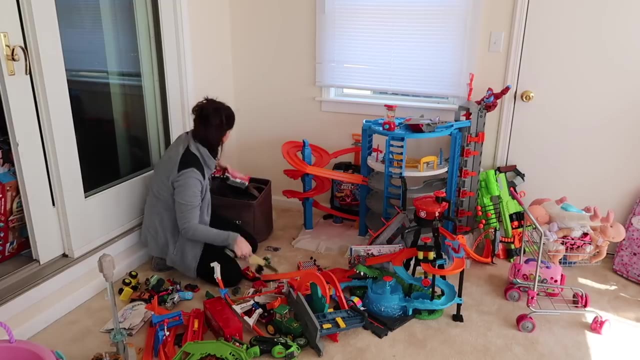 But you know it's not about our love fading. You know it's not about. Yeah, you know it's not about our love ending. You know it's not about. You know it's not about. It's not about us. You know it's not about us. 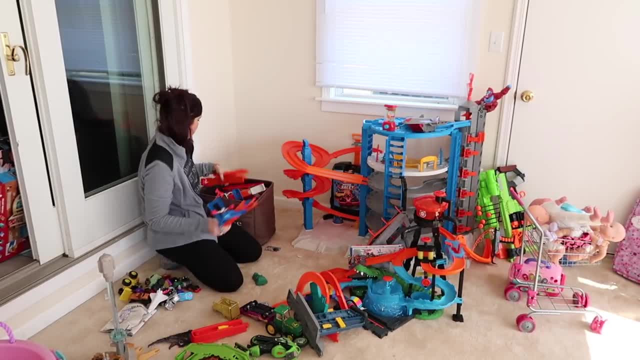 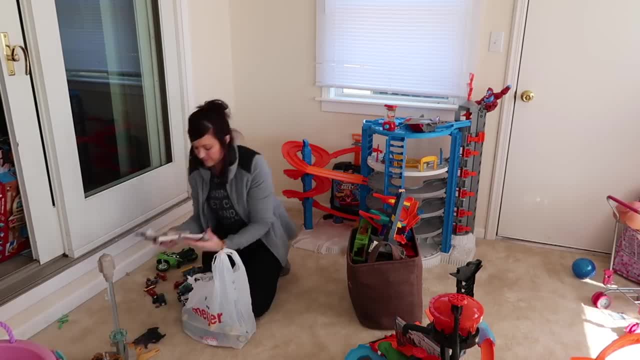 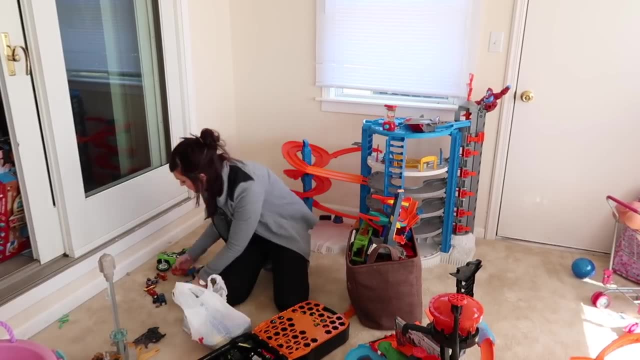 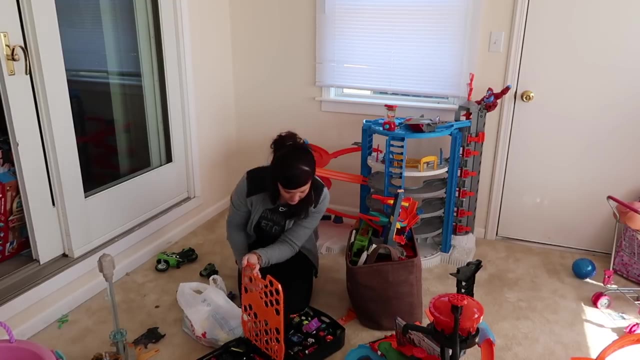 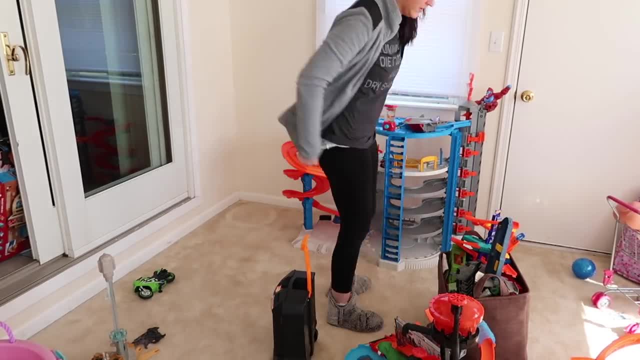 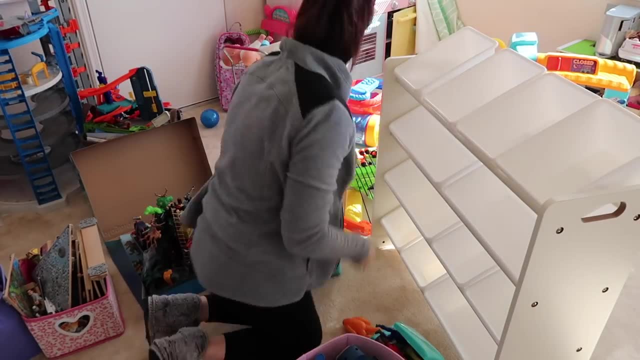 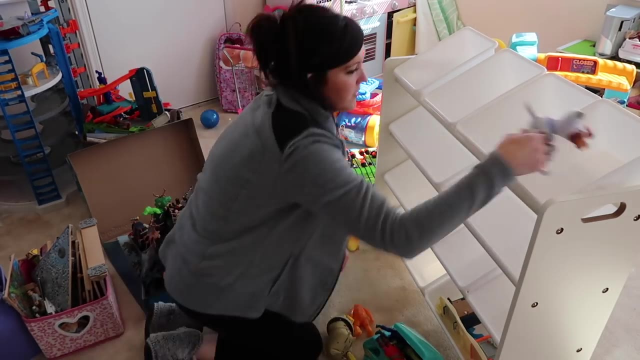 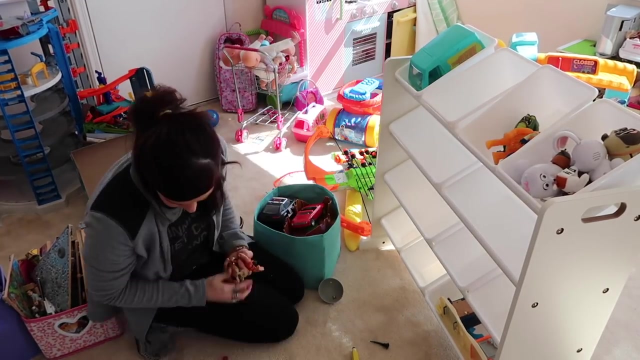 You always pick me up When I am down. It's like you have a spark That leaves me burning. You say all the right things. You just have your ways To get me high. You make all my dreams come true. It feels right When I'm around you. We can break up. And then make up. I always come back to you. You move me in a way Never thought anyone could you Get me high. You're my drug When I am feeling blue. Yeah, You make all my dreams come true. You just have your ways. It's all you Cause. you're the one. 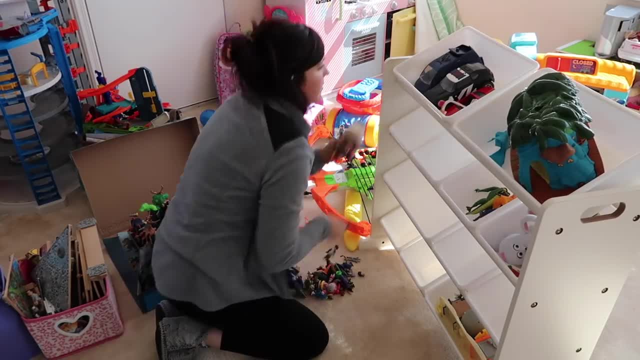 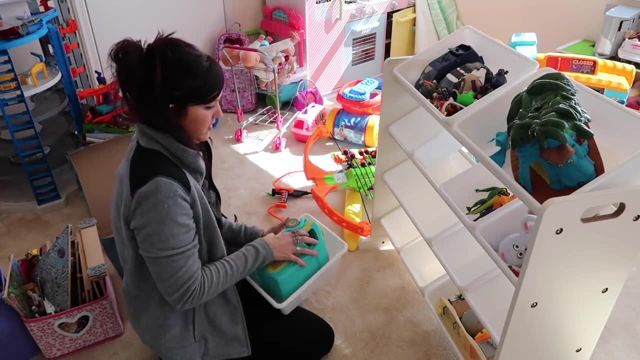 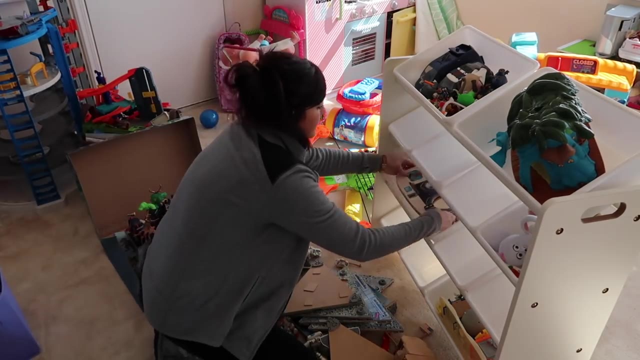 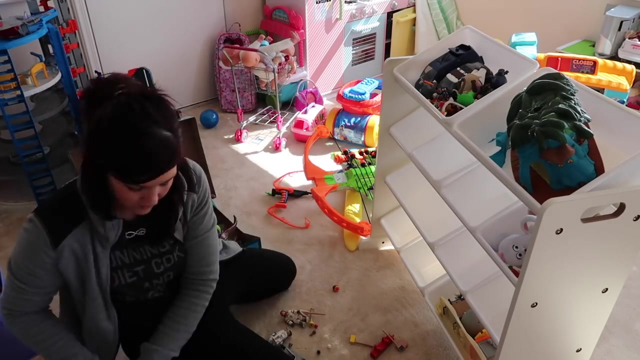 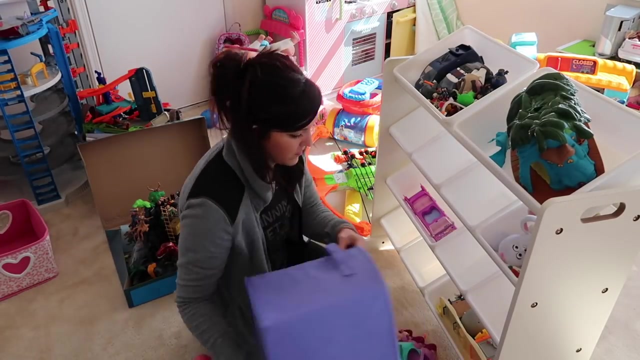 Yeah, the one. Yeah, you're the one, Yeah, the one. You touch me in a way That makes me shiver. Sometimes I can't believe That you are mine. Love's a gun and baby. You're my dream Girl. you kiss me In a way that gets me high. 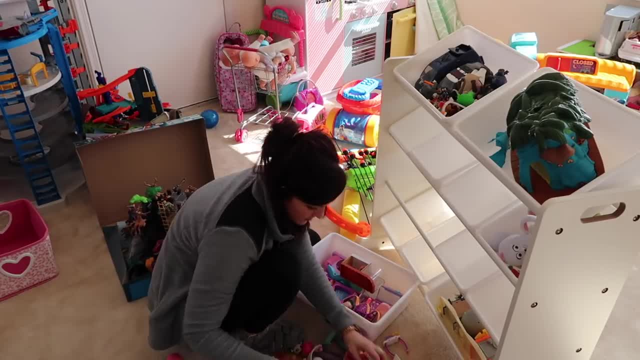 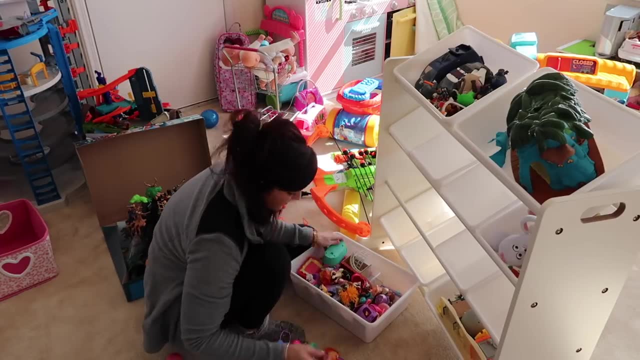 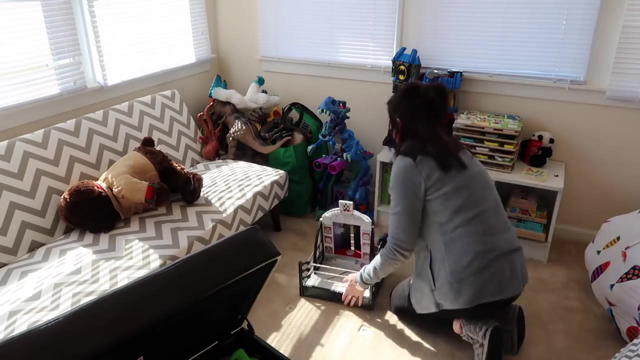 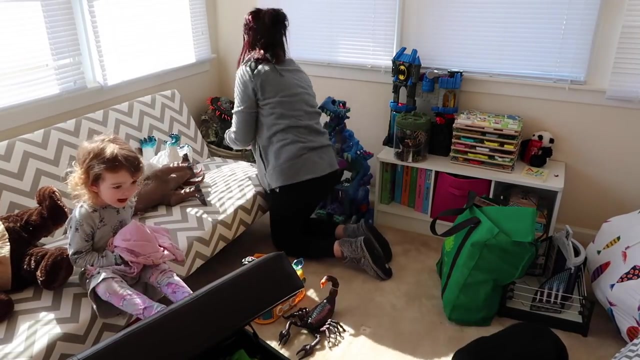 You make all my dreams come true. It feels right Just being around you. We can break up And then make up. I always come back to you. You move me in a way Never thought anyone could you Get me high. You're my drug When I am feeling blue. 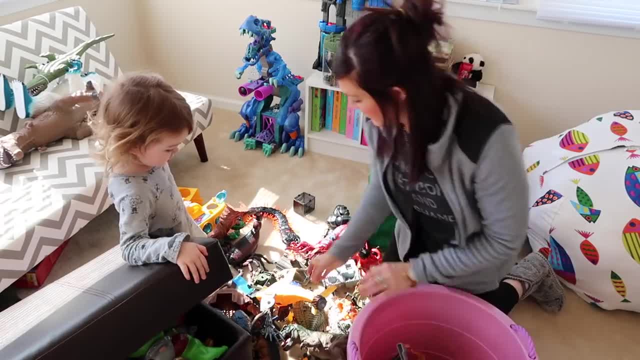 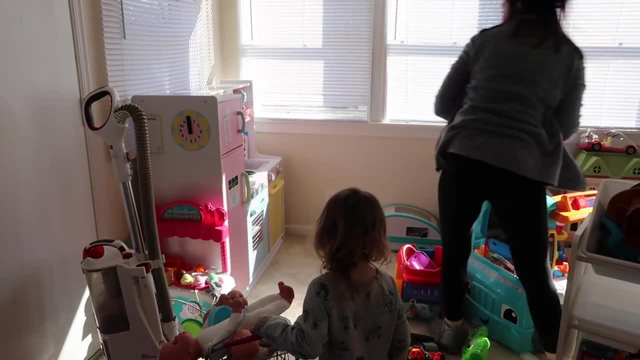 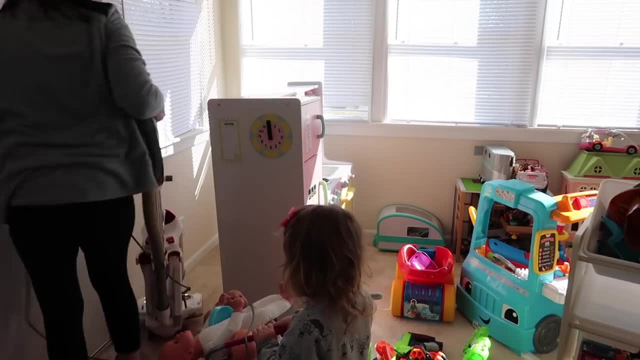 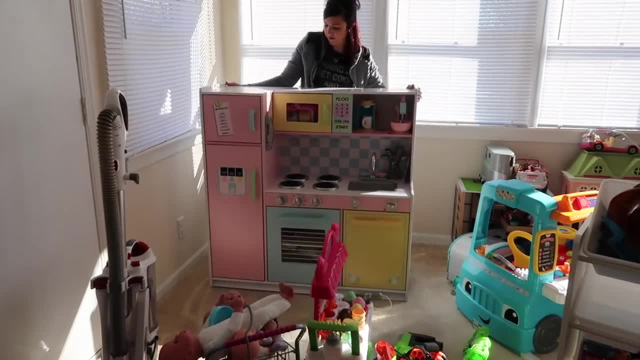 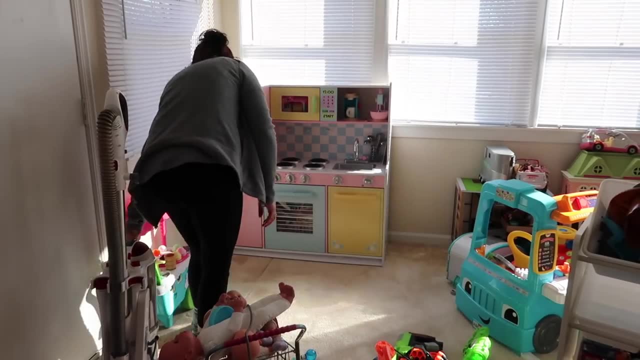 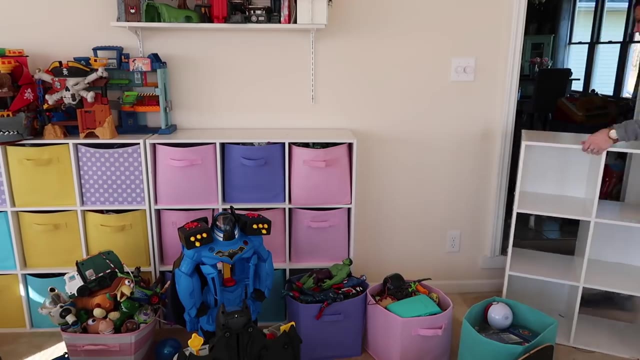 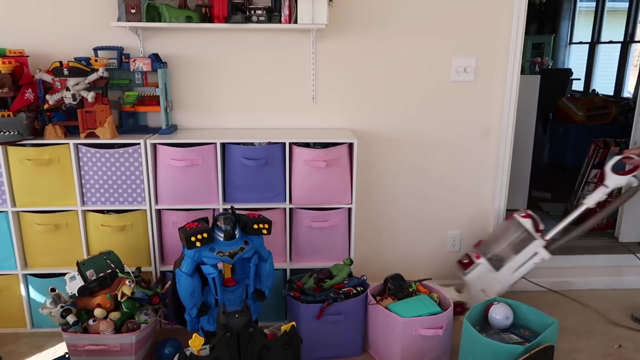 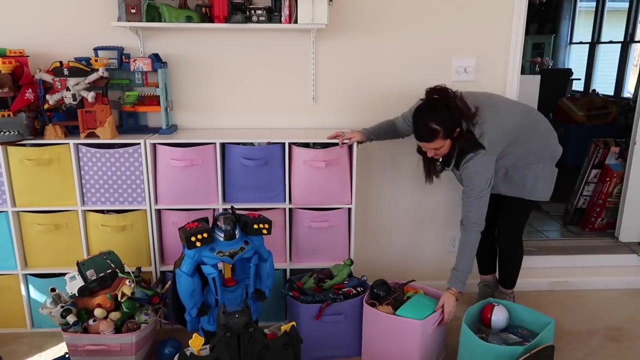 Yeah, you're the one. Come back, Yeah, you, you, you You're the one. Cause you're the one, Yeah, the one. Yeah, you're the one. Yeah, the one, Cause you're the one. Yeah, the one. Yeah, you're the one, yeah, the one. 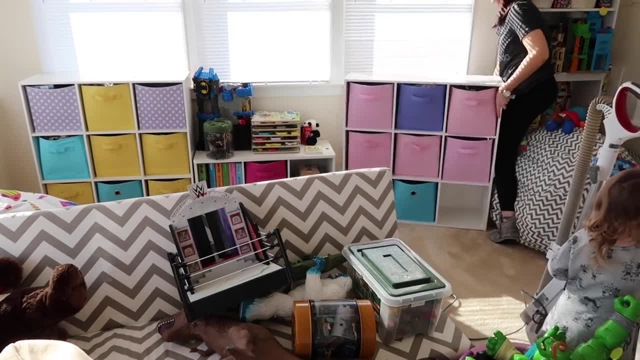 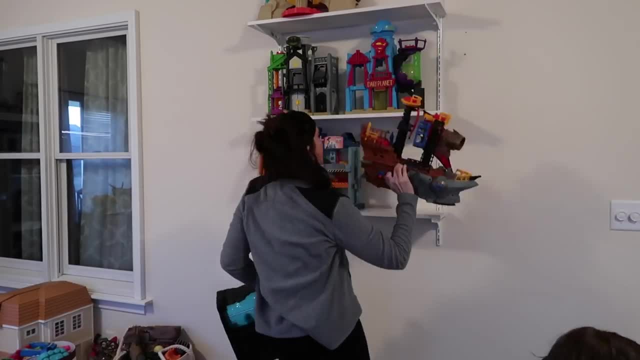 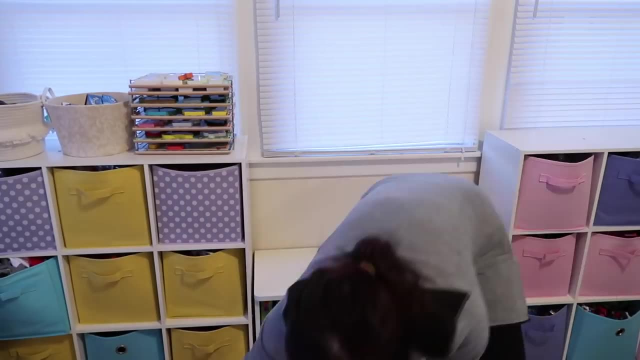 Funny how the story goes: little hope but bigger dreams. Ah, they try to bring a sucker down singing louder than the crowd. Ah, listen to the rhythm. I'm feeling brand new. Can't push it forward, it's gonna save you. 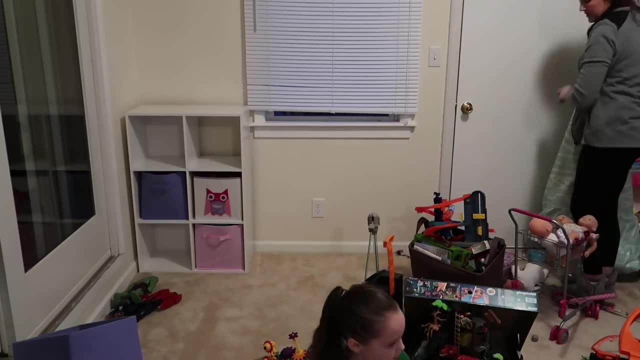 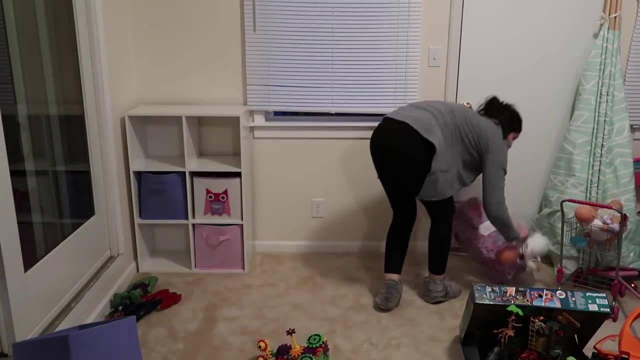 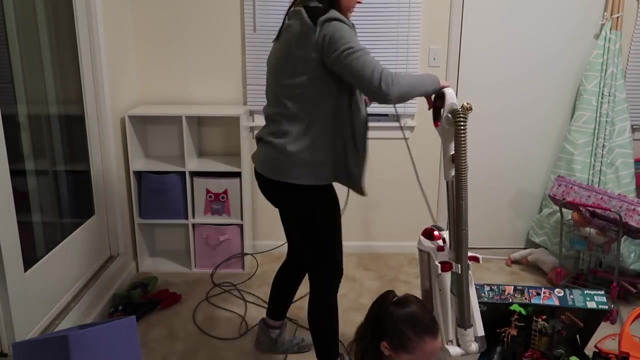 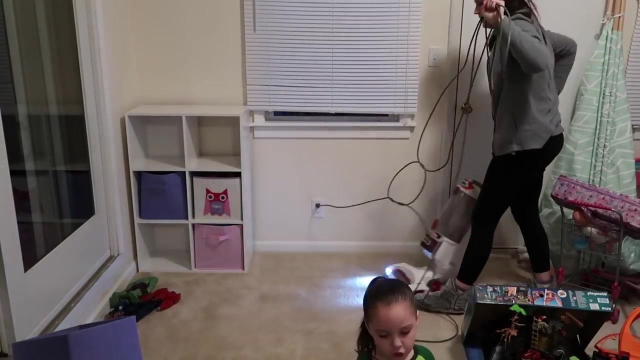 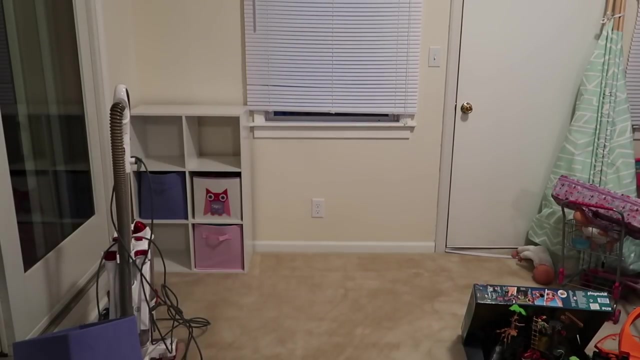 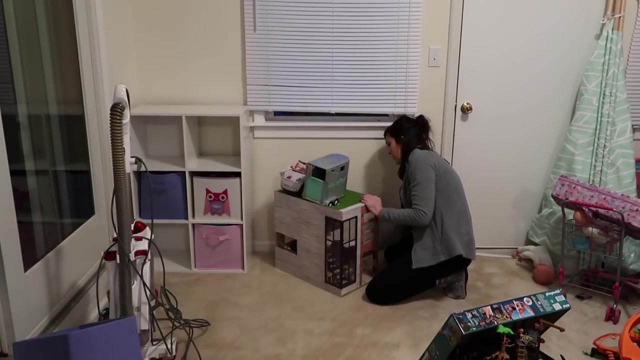 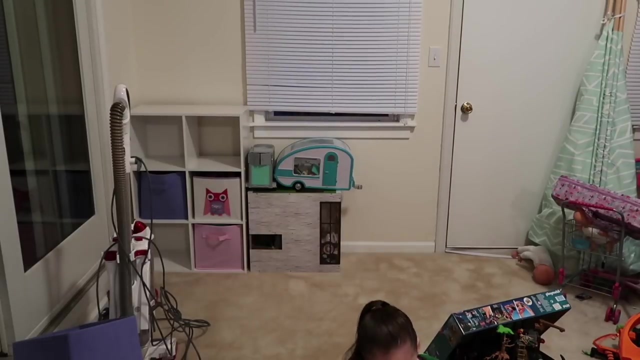 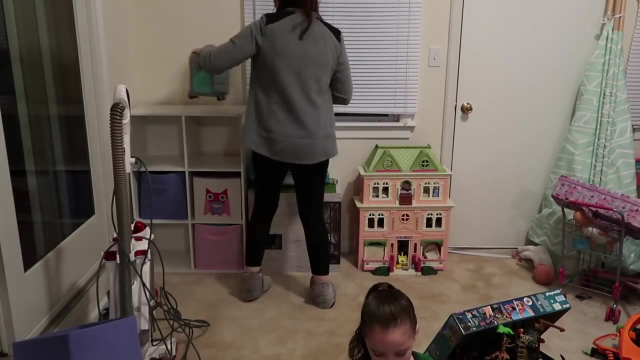 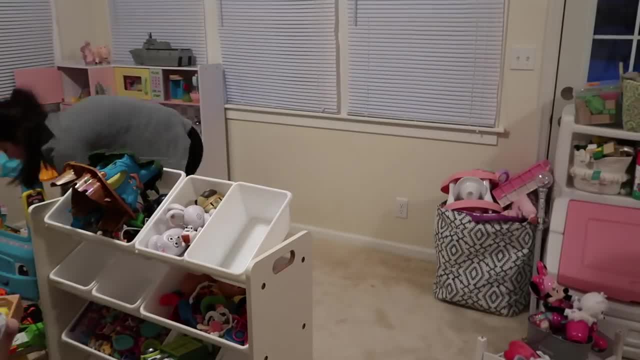 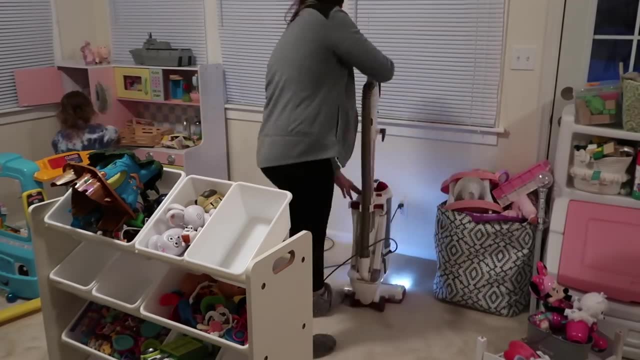 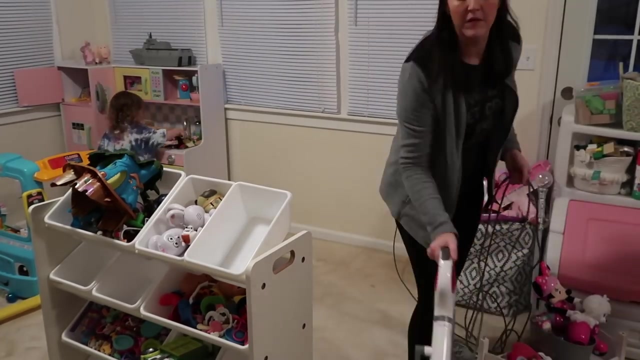 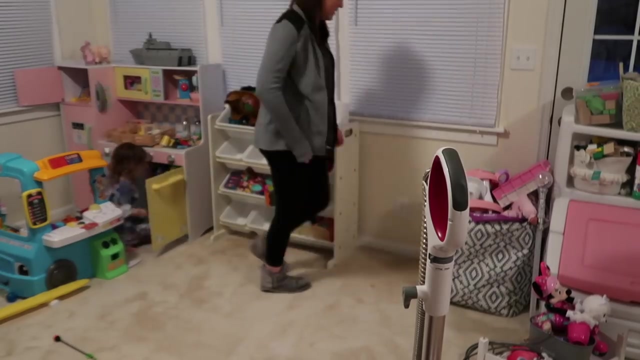 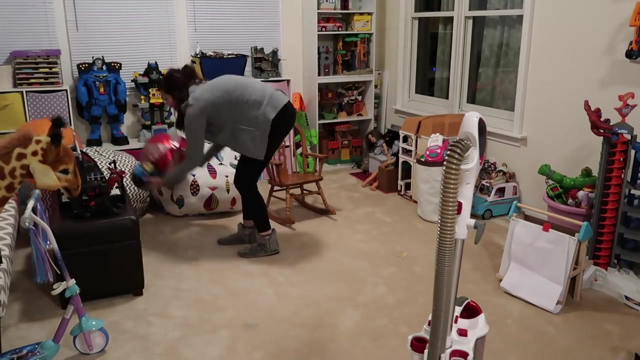 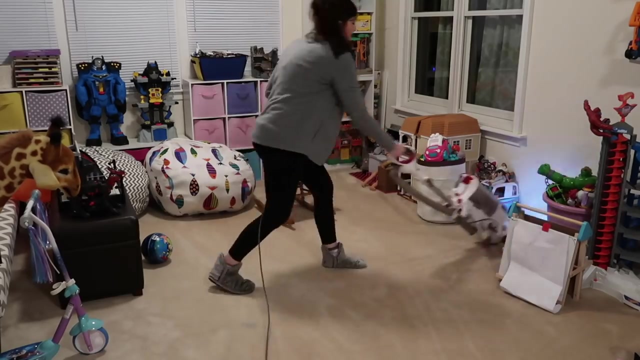 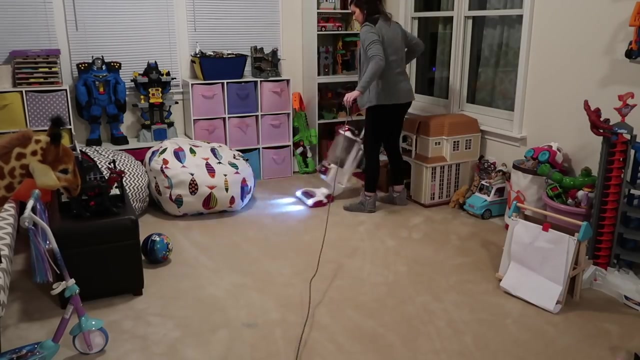 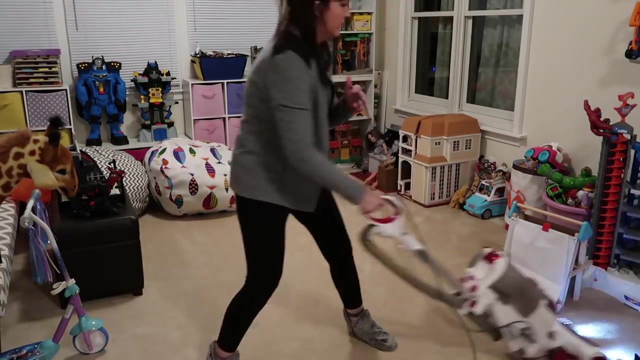 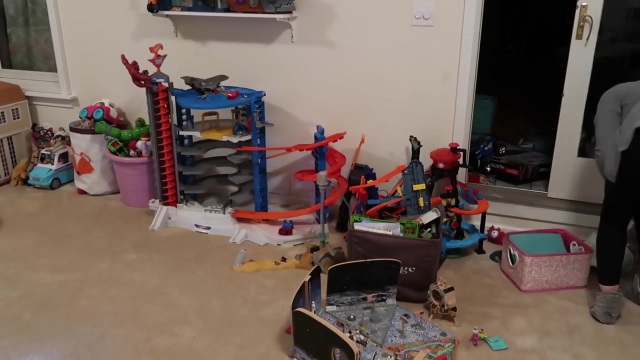 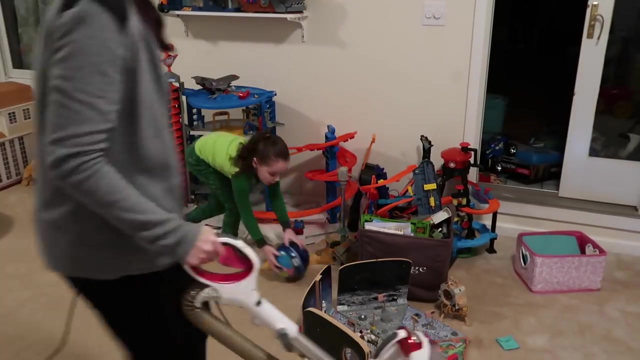 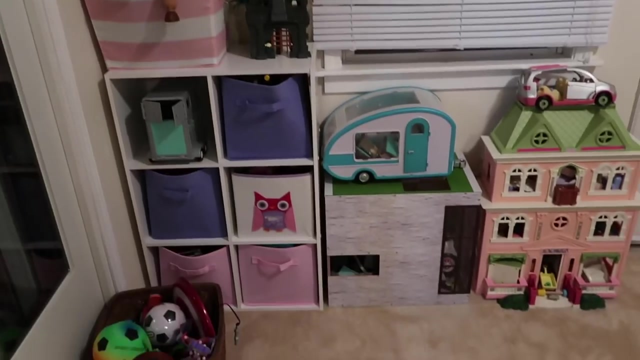 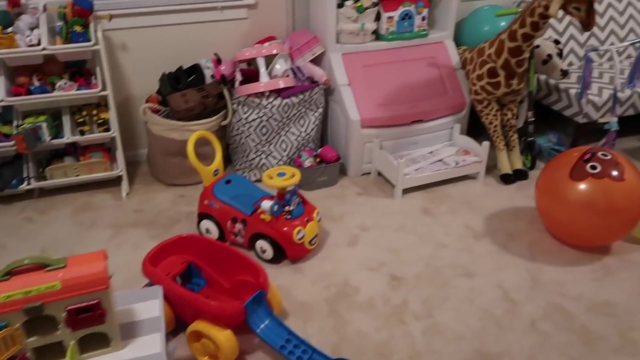 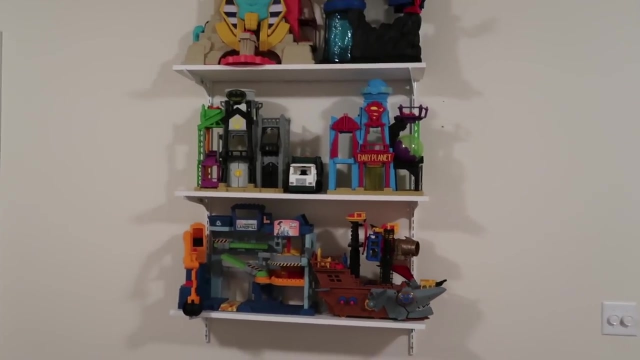 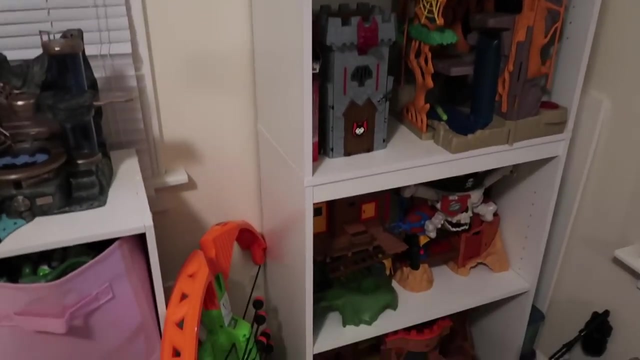 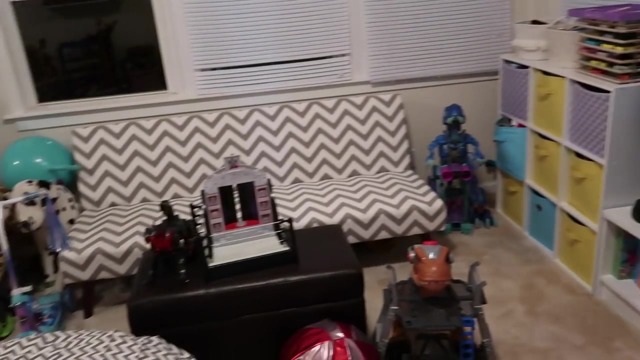 ah, ah ah. the sun is getting warmer. but when we store our way among the clouds, this time it's just a border, but when we're floating up like helium, We'll be right back. Never up, never down, never Like a theme in a song.